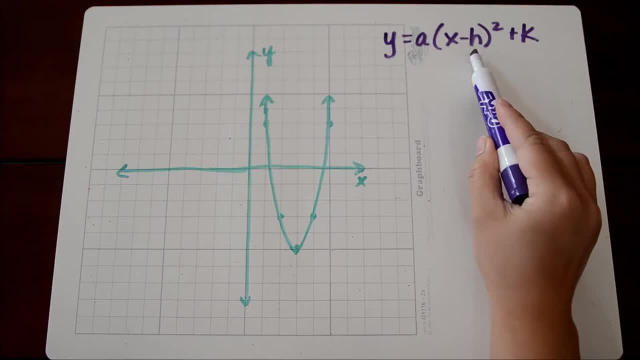 are the vertex, because that will be our h and our k value, as well as some other point on our graph that we'll substitute in for the x and y values. The a value is the missing value. That is what we are supposed to solve for. 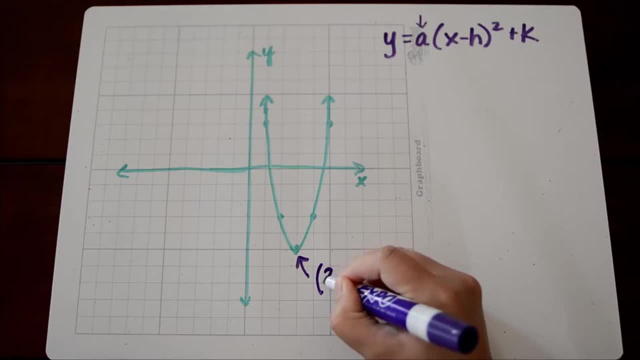 So let's start with our vertex Here. the vertex of this parabola is 3, negative 5, which means h is 3, and k is negative 5.. And let's just choose this point on our graph. This point is 4, negative 3.. That will be substituted in for x and y. 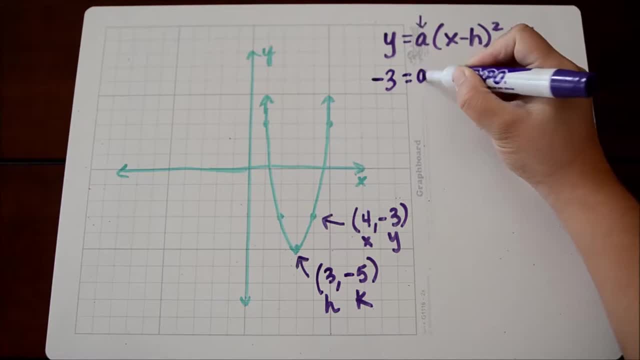 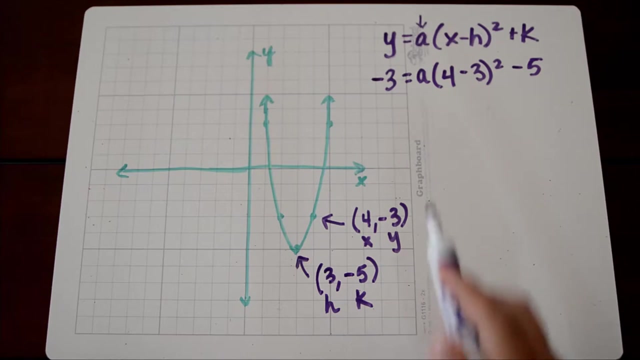 So we'll write negative: 3 equals a times 4 minus 3, squared minus 5.. We're going to use order of operations to simplify. So 4 minus 3 is 1.. 1 squared is still 1.. So let's write negative: 3 equals 1a minus 5.. And then we have a two-step equation. 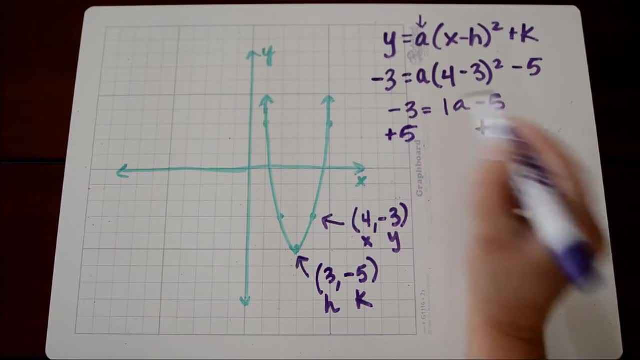 We're going to use inverse operations to solve, So we'll add to zero out the constant and then we get 2 equals 1a, and then we'll divide to get a by itself And we're left with a equals 2.. So that tells us what our a value is. 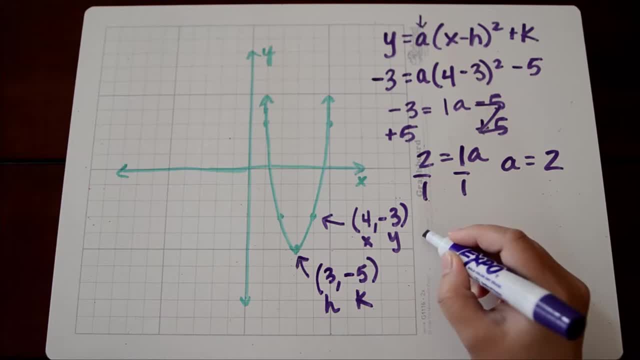 but we still have to substitute it back into vertex form. So our answer is: y equals 2 times x minus 3, squared minus 5.. We don't substitute back our x and our y values. Let's take a look at one more example. 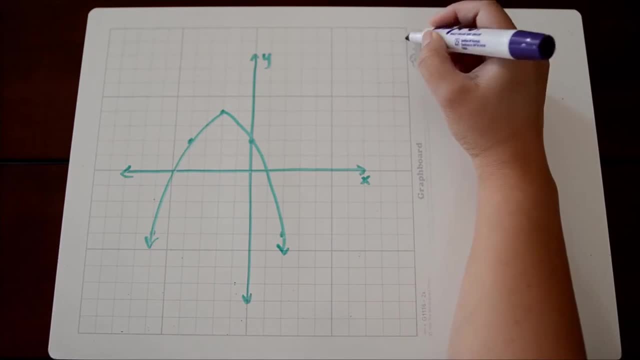 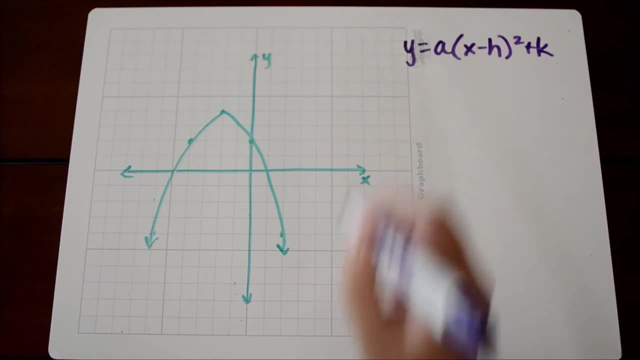 So again, I'm going to write vertex form so I could show you where we're going to substitute in all our values. Let's start first by identifying our vertex. The vertex of this graph is negative, 2, 4. And let's choose this point, This will be our x and our y value.